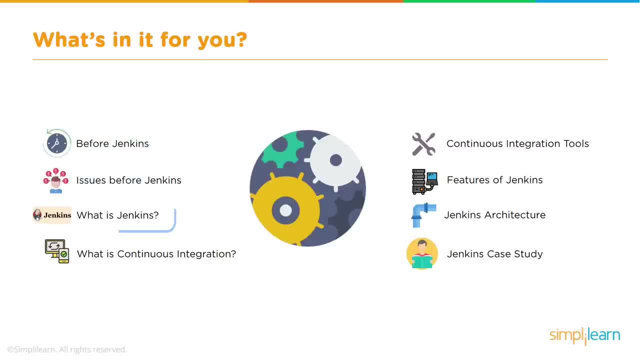 issues that Jenkins specifically addresses. Then we'll get into what Jenkins is about and how it applies to continuous integration and the other continuous integration tools that you need in your DevOps team. Then, specifically, we'll deep dive into features of Jenkins and the Jenkins architecture and we'll give you a case study of a company that's using Jenkins today to actually 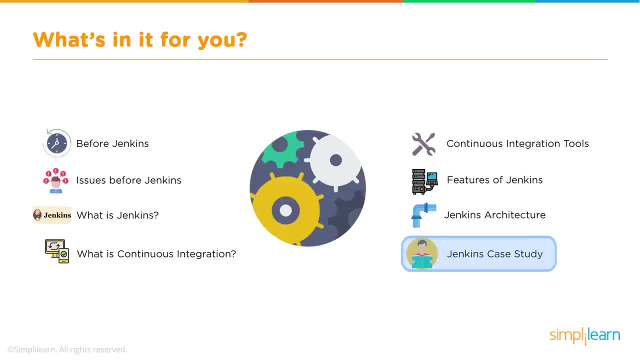 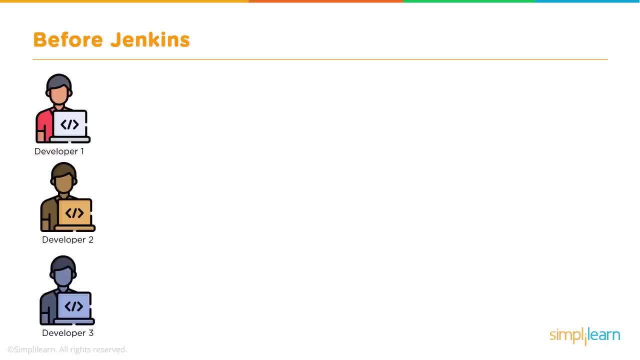 transform how their IT organization is operating. So let's talk a little bit about life before Jenkins. Let's see this scenario. I think it's something that maybe all of you can relate to As developers. we're going to be talking about how life is like before we use Jenkins. 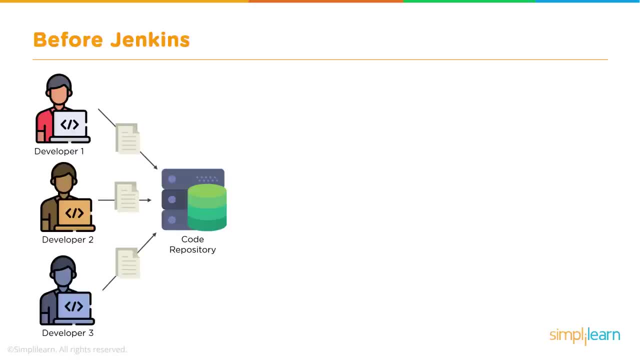 As developers, we all write code and we all submit that code into a code repository and we all keep working away writing our unit tests and hopefully we're running our unit tests, But the problem is that the actual commits that actually get sent to the code repository aren't consistent. You, as a 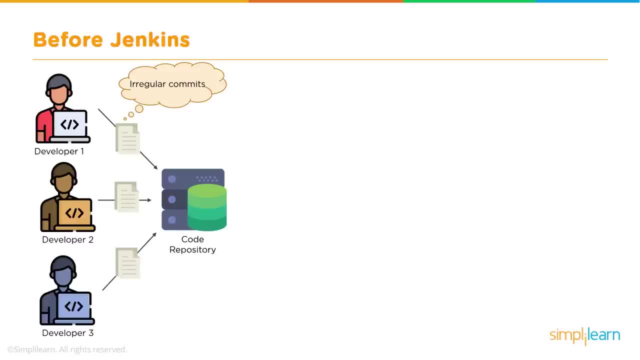 developer may be based in India, you may have another developer that's based in the Philippines, and you may have another team lead that's based in the UK and another development team that's based in North America. So you're all working at different levels of development. You're all working at 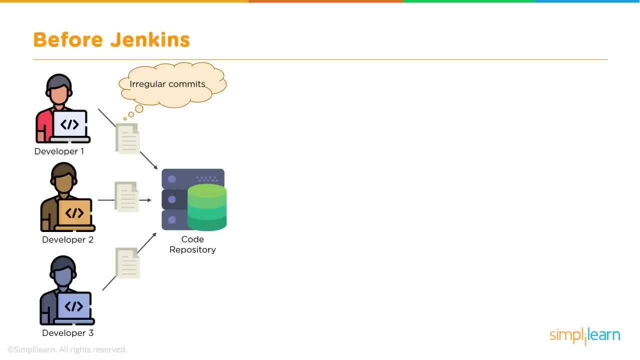 different times and you have different amounts of code going into the code repository. There's issues with integration and you're kind of running into a situation that we'd like to call development hell, where things just aren't working out and there's just lots of delays being added into the project. 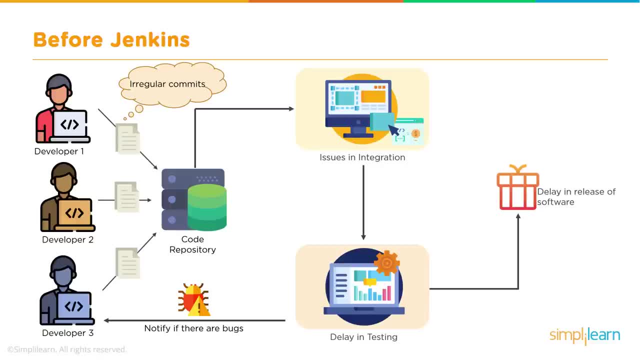 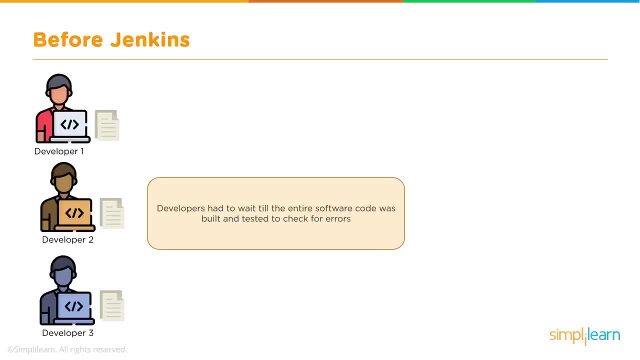 and the bugs just keep mounting up. The bottom line is the project is delayed, And in the past, what we would have to do is we'd have to wait until the entire software code was built and tested and built. So we'd have to wait until the entire software code was built and tested, and 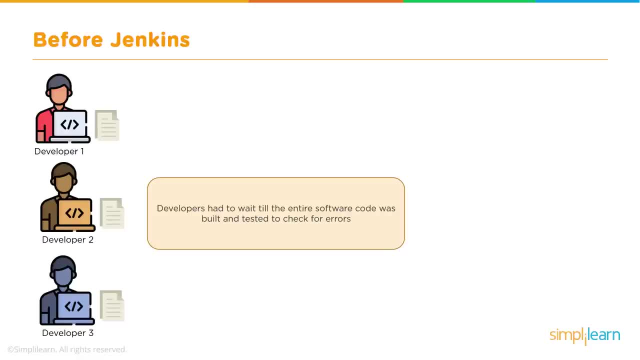 before we could even begin checking for errors, And this just really kind of increased the amount of problems that you'd have in your project. The actual process of delivering software was slow. There was no way that you could actually iterate on your software, And you just ended up with just 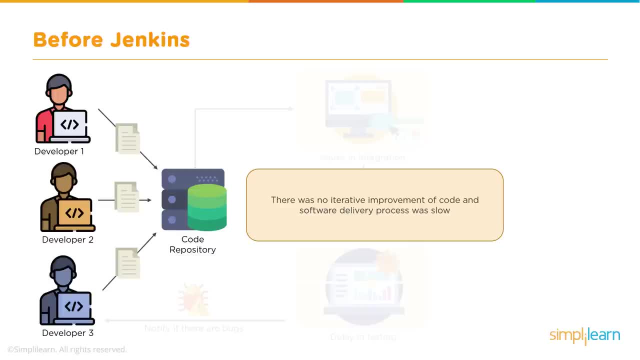 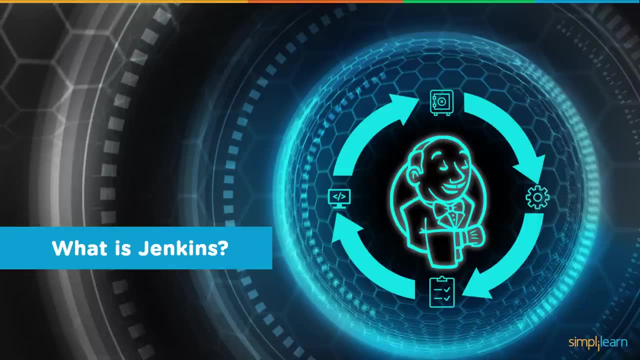 a big headache, with teams pointing fingers at each other and blaming each other. So let's jump into Jenkins and see what Jenkins is and how it can address these problems. So Jenkins is a project that's based in the UK. It's a project that's based in the UK. It's a project that's based 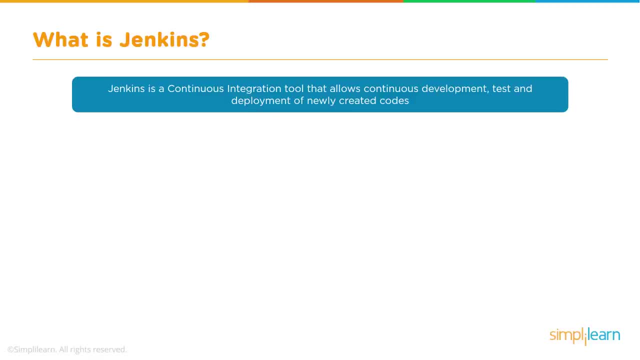 in the UK. It's a product that comes out of the concept of continuous integration that you may have heard of as power developers, where you'd have two developers sitting next to each other coding against the same piece of information. What they were able to do is to continuously develop their 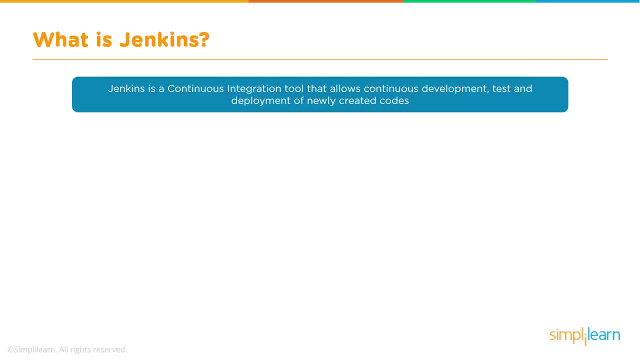 code and test the code and move on to new sections of code. Jenkins is a product that allows you to expand on that capacity to your entire team, So you're able to submit your codes consistently into a source code environment. You're able to submit your codes consistently into a source code environment. 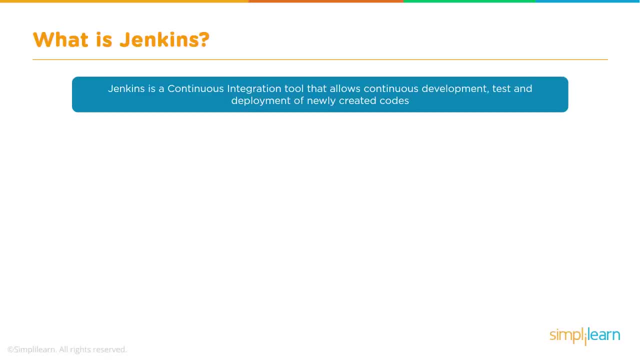 So there are two ways in which you can do continuous delivery. One is through nightly builds and one is through continuous. So the approach that you can look at continuous delivery is modifying the legacy approach to building out solutions. So what we used to do is we would wait for nightly builds And the 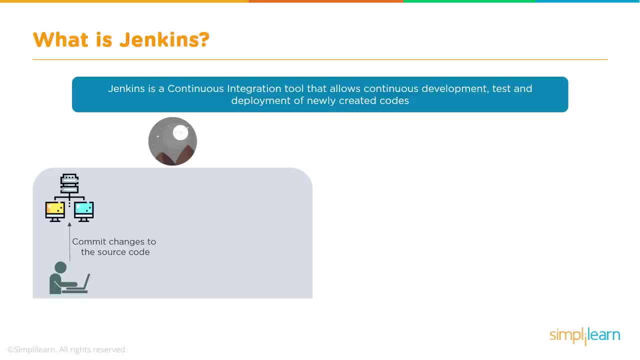 way that our nightly builds would work and operate is that, as code developers, we would all run and have a cutoff time at the end of the day that was consistent around the world, that we would put up our codes into a single repository And at night all of that code would be run and operated and tested to see if 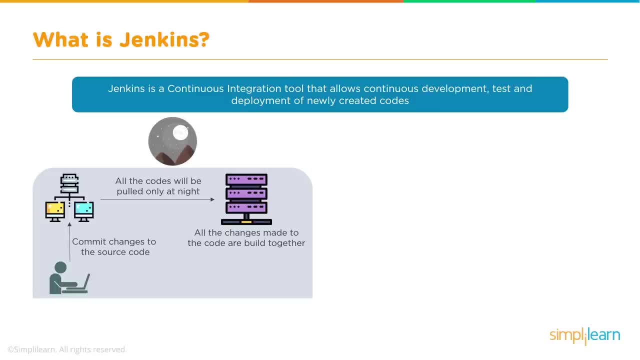 there were any changes and a new build would be created, And that would be referred to as the nightly build. With continuous integration, we're able to go one step further. We're able to not only commit our changes into our source code, but we can actually do this continuously. There's no need to race and have a team get all of their. 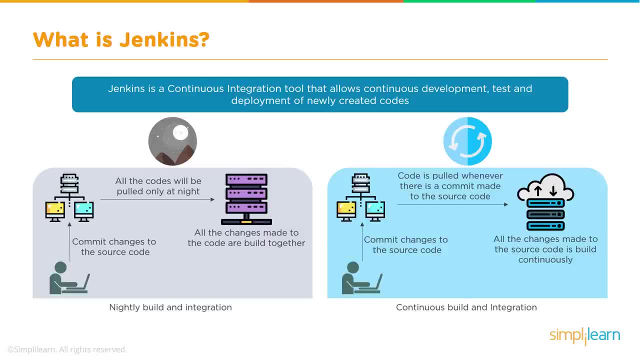 code in at an arbitrary time. You can actually do a continuous release, because what you're doing is you're putting your tests and your verification services into the build environment, So you're always running cycles to test against your code. This is the power that Jenkins provides in. 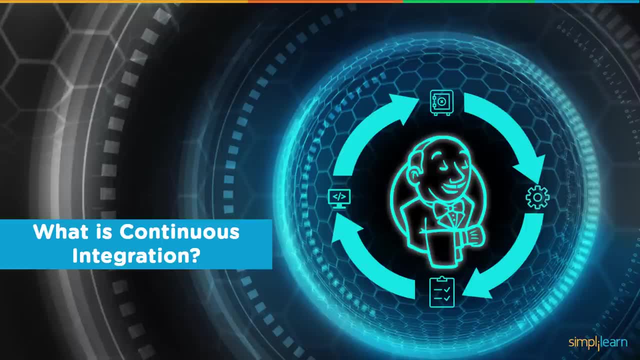 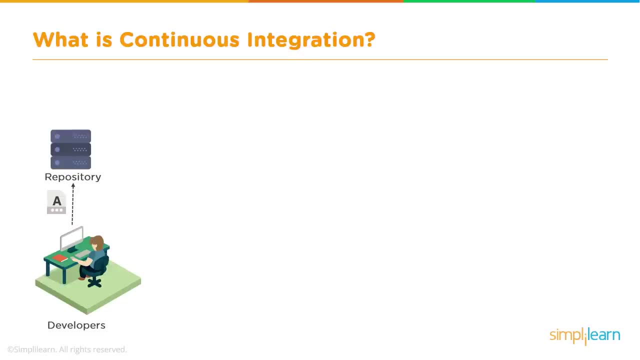 continuous integration. So let's dig deeper into continuous integration. So the concept of continuous integration is that, as a developer, you're able to pull from a repository the code that you're working on and then you'll be able to then, at any time, submit the code that you're working on into a continuous integration. 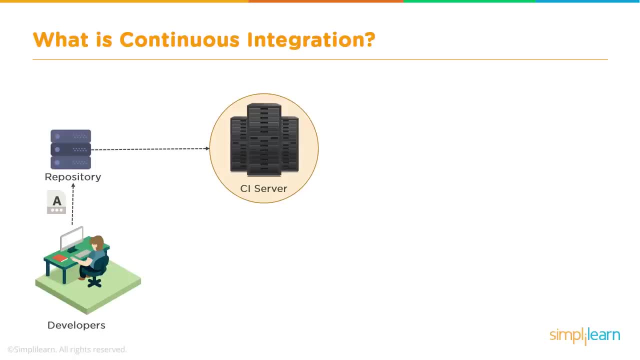 server And the goal of that continuous integration server is that it actually goes ahead and validates and passes any tests that a tester may have created. Now, if on the continuous integration server a test isn't passed, then that code gets sent back to the developer and the developer can then make the changes. It allows the developer to actually do a 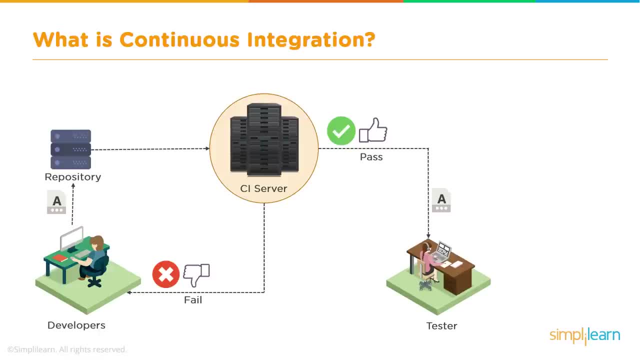 couple of things. It allows the developer not to break the build- and we all don't want to break the builds that are being created- but it also allows the developer not to actually have to run all of the tests locally on their computer Running tests, particularly if you have a large number of 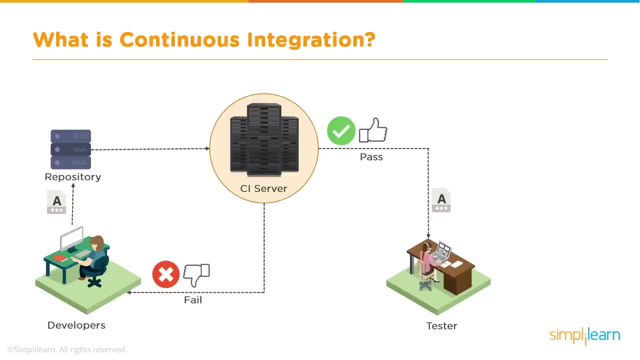 tests can take up a lot of time, So if you can push that service up to another environment like a continuous integration server, it really improves the productivity of your developer. What's also good is that if there are any code errors that have come up, that may be beyond just the 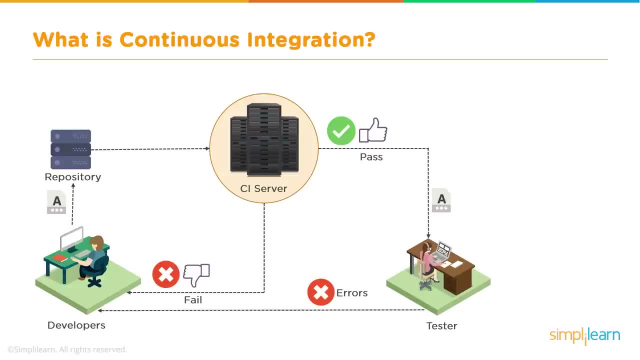 standard CI tests. so maybe there's a code. the way that you write your code isn't consistent. those errors can then be passed on easily from the tester back to the developer too. The goal from doing all this testing is that you're able to release and deploy, and your 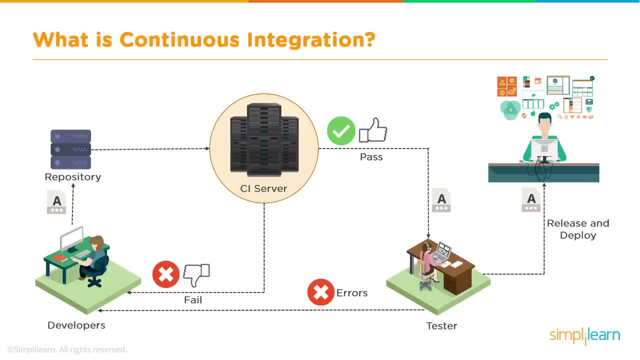 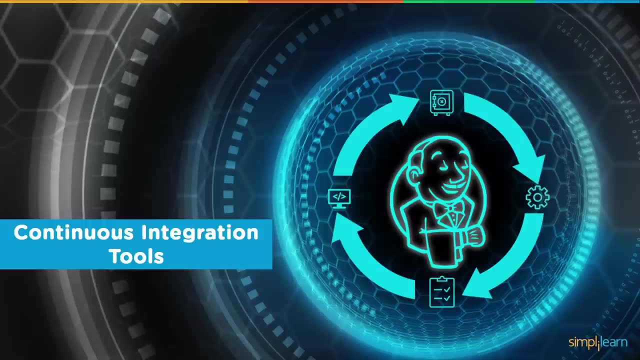 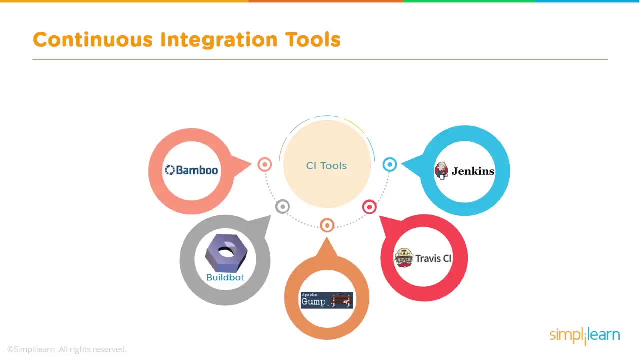 customer is able to get new code faster, and when they get that code, it simply just works. So let's talk a little bit about some of the tools that you may have in your continuous integration server. Just a quick way to put this in perspective: you can use the continuous integration environment. So the cool thing with working with 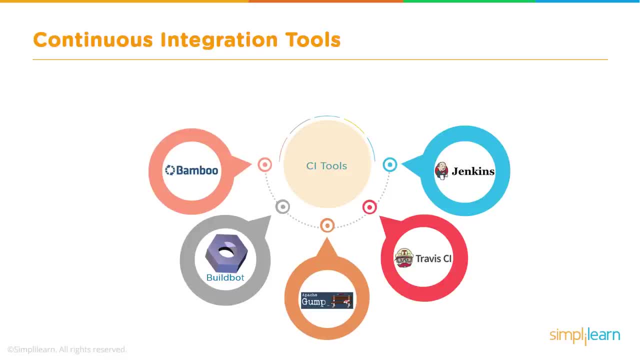 continuous integration tools is that they are all open-source, or at least the ones that we have listed here are all open-source. There are some that are private, but typically you'll get started with open-source tools and it gives you the opportunity to 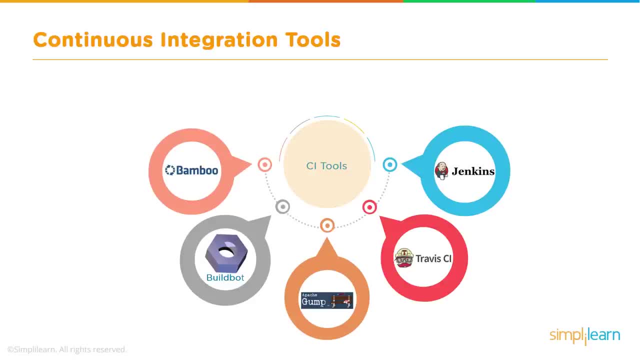 understand how you can accelerate your environment quickly. So Bamboo is a continuous integration tool that specifically runs multiple builds in parallel for faster compilation. So if you have multiple builds in parallel but you can maintain them, these tools are very, very easy to use. but they are also very, very difficult to use, so you can use them in your own way. That's why I've got this tool, the Bamboo 5U4002,. 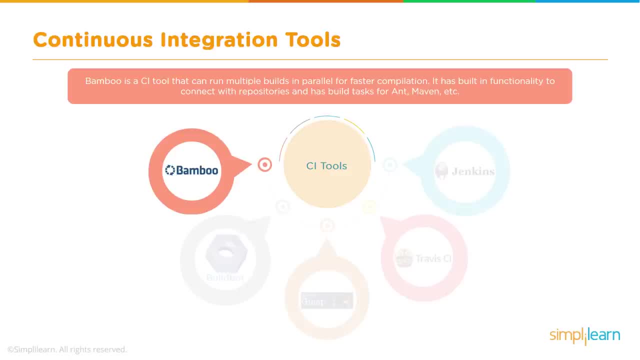 So if you have multiple versions of your software that runs on multiple platforms, this is a tool that really allows you to get that up and running super fast so that your teams can actually test how those different builds would work for different environments. And this has integration with Ant and Maven and other similar tools. 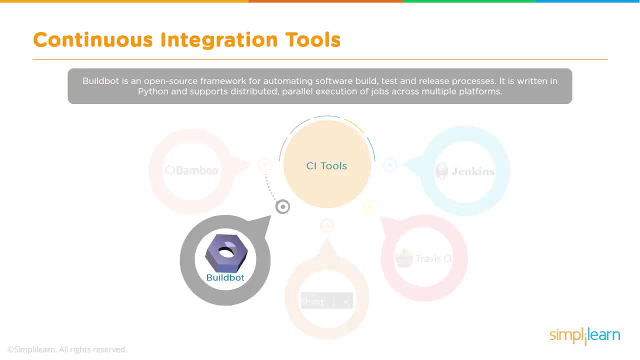 So one of the tools you're going to need is a tool that allows you to automate the software build, test and release process, And BuildBot is that open source product for you. Again, it's an open source tool, so there's no license associated with this. 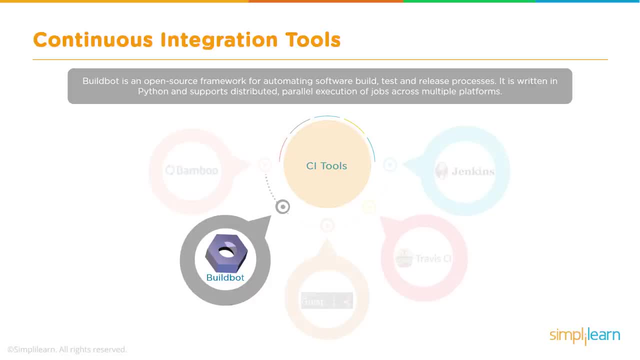 So you can actually go in and you can actually get the environment up and running and you can then test for and build your environment and create releases very quickly. So BuildBot is also written in Python and it does support parallel execution jobs across multiple platforms. 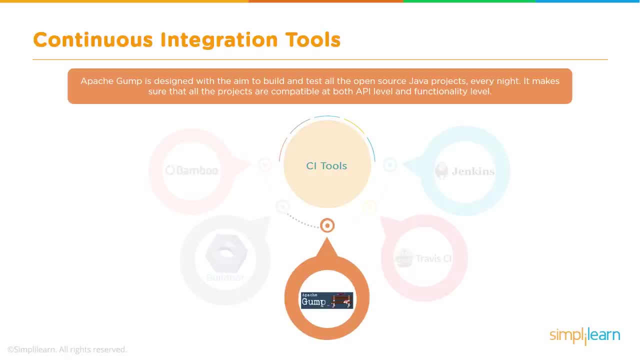 If you're working specifically on Java projects that need to be built and test, then Apache Gump is the tool for you. It makes all of those projects real. It's really easy. it makes all the Java projects easier for you to be able to test, with API level and functionality level testing. 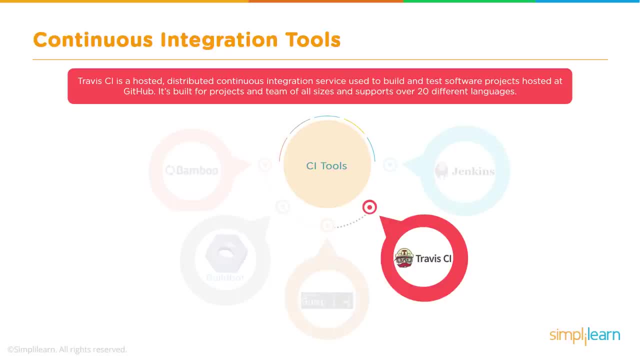 So one of the popular places to actually store code and create a version of your code is GitHub, And it's a service that's available on the web just recently acquired by Microsoft. If you are storing your projects in GitHub, then you'll be able to use Travis Continuous Integration or Travis CI. 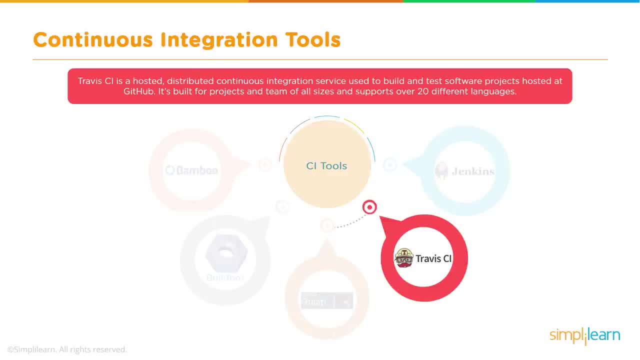 And it's a tool designed specifically for hosted development, And you can actually bring in Kotlin to your localorer and use that to build GitHub projects, And so finally, we're covering Jenkins, And Jenkins is a central tool for automation for all of your projects. 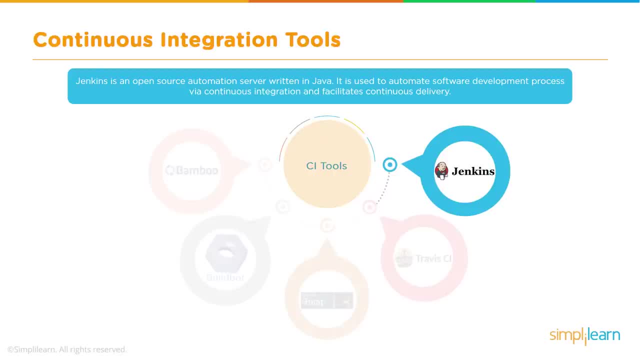 Now, when you're working with Jenkins, sometimes you'll find there's documentation that refers to a product called Hudson. Hudson is actually the original version of the product that finally became Jenkins, And it was acquired by Oracle. When that acquisition happened, the team behind Hudson was a little concerned about the data. 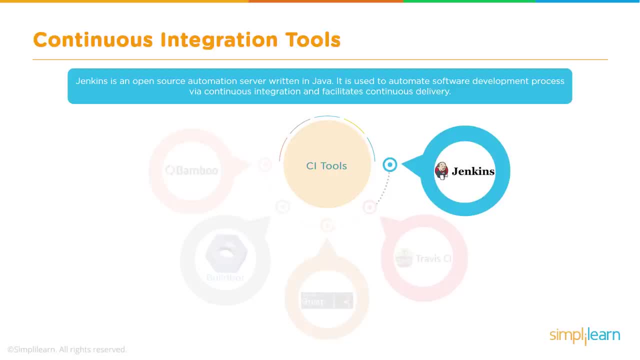 direction that Oracle may potentially go with Hudson, and so they created a hard fork of Hudson that they renamed Jenkins, and Jenkins has now become that open-source project. it is one of the most popular and continuously contributed projects that's available as open source, so you're always getting new. 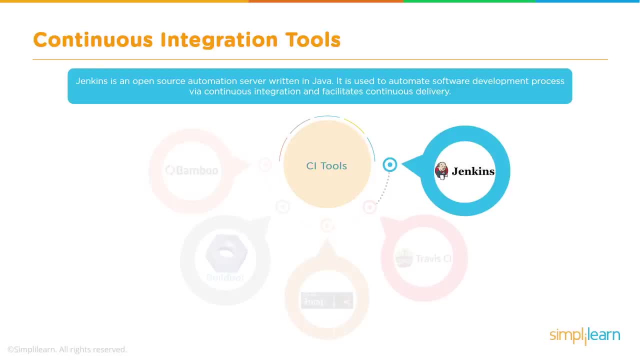 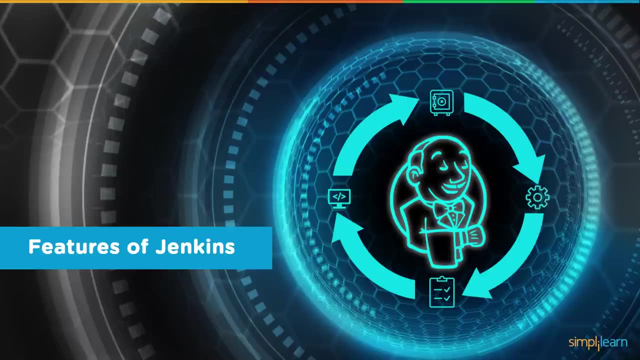 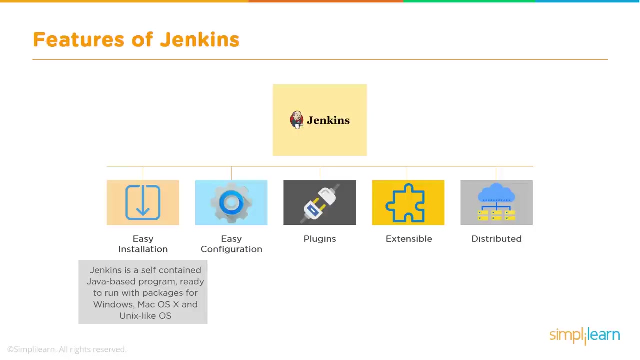 features being added to it. it's a tool that really becomes the center for your CI environment. so let's jump into some of those really great features are available in Jenkins. so Jenkins itself is really comprised of five key areas around: easy installation, easy configuration, plugins, extensibility and 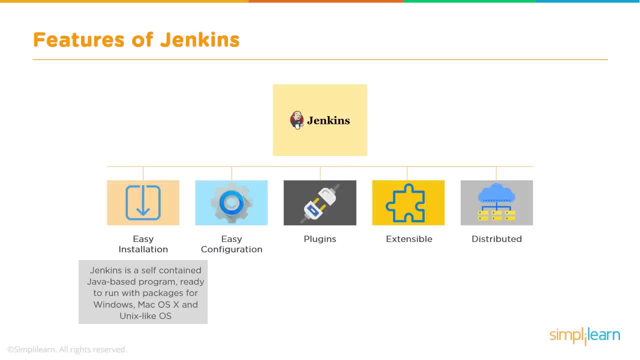 distribution. so, as I mentioned for the easy installation, Jenkins is a self-contained Java program and that allows it to run on most popular operating systems, including Windows, Mac OS and Unix. you even run it on Linux. it really isn't too bad to set up. it used to be a little bit of a pain in the ass. 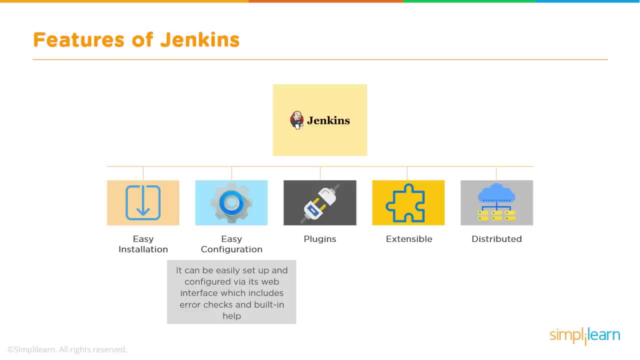 to be much harder than it is today. the setup process has really improved. the web interface makes it really easy for you to check for any errors. in addition, you have great built-in help- one of the things that makes tools like Jenkins really powerful for developers and continuous integration teams- and your 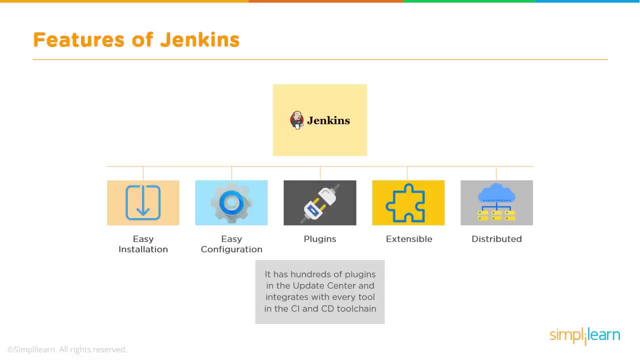 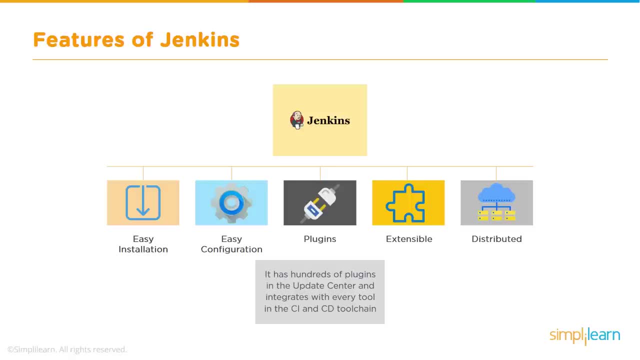 and see which other plugins that would be good for your DevOps environment. certainly check it out. there's just lots of stuff out there. in addition to the plugin architecture, Jenkins is also extremely extensible. the opportunity for you to be able to configure Jenkins to fit in your environment is almost. 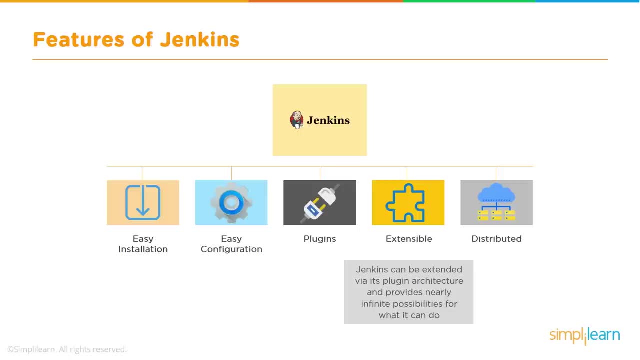 endless. now it's really important to remember that you are extending Jenkins, not creating a custom version of Jenkins, and that's a great difference, because the core foundation remains as the core Jenkins product. the extensibility can then be continued with newer releases of Jenkins, so you're. 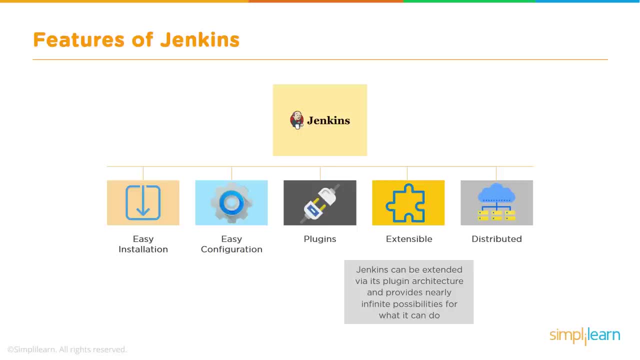 always having the latest version of Jenkins and your extensions mature with those core foundation. the distribution and the nature of Jenkins makes it really easy for you to be able to have it available across your entire network. it really will become the center of your CI environment and it's certainly one of the 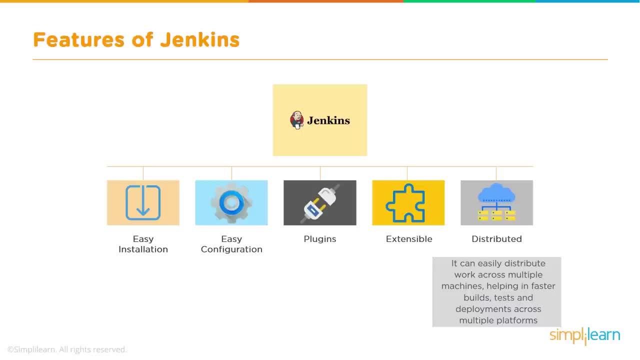 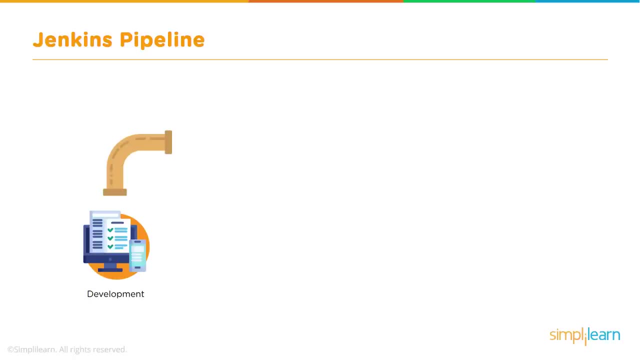 easier tools and more effective tools for DevOps. so let's jump into the standard Jenkins pipeline. so when you're doing development, you start off and you're coding away on your computer, the first thing you have to do when you're working in the Jenkins pipeline is to actually commit your code now as a 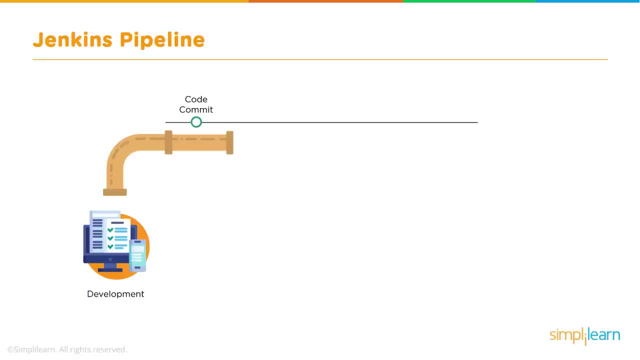 developer. this is something that you're already doing, or at least you should be doing. you're committing your code to a git server or to an SVN server or a similar type of service, so in this instance, you'll be using Jenkins as the place for you to commit your code. Jenkins will then create a. 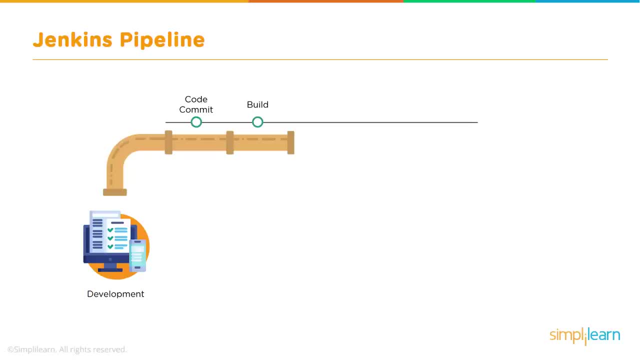 build of your code and part of that build process is actually going through and running through tests and, as again, as a developer, you're already comfortable with running unit tests and writing those tests to validate your code. but there may be additional tests that Jenkins is running. so, for instance, 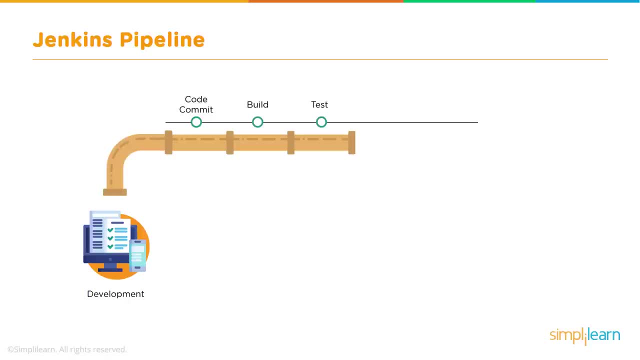 as a team, you may have a standard set of tests for how you actually write out your code, so that each team member can understand the code that's been written, and those tests can also be included in the testing process within the Jenkins environment. assuming everything passed the tests, you can then get everything placed in a stage and 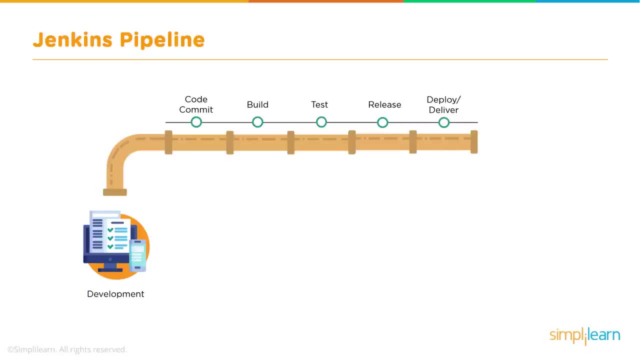 release ready environment within Jenkins and, finally, getting ready to deploy or deliver your code to a production environment. Jenkins is going to be the tool that helps you with your server environment to be able to deploy your code to the production environment, and the result is that you're able to move from a developer to production code. 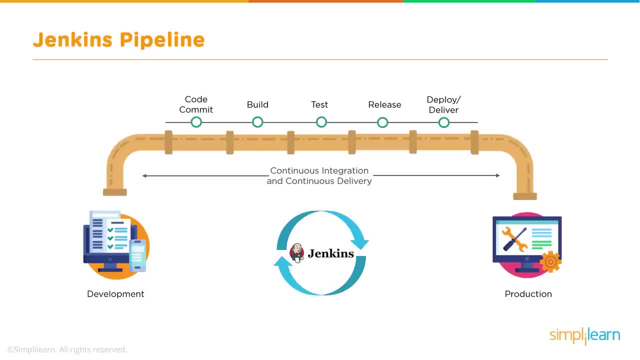 really quickly. this whole process can be automated. rather than having to wait for people to actually test your codes or going through a nightly build, you're looking at being able to commit your code and go through this testing process and release process continuously. as an example, companies Etsy will release up. 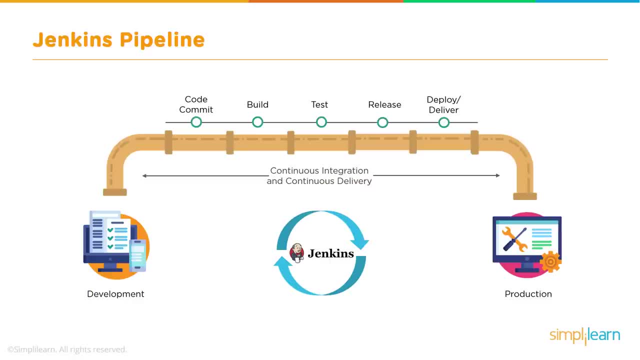 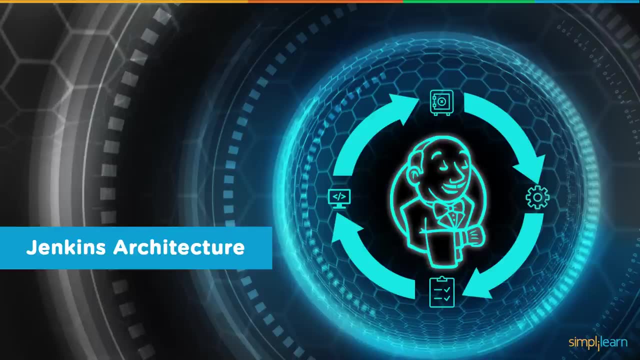 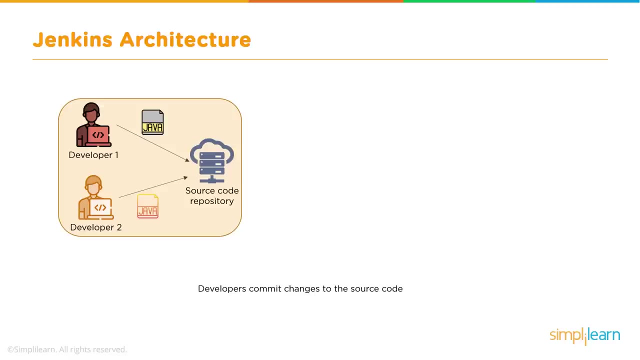 to 50 different versions of their website every single day. so let's talk about the architecture within Jenkins that allows you to be so effective at applying a continuous delivery DevOps environment. so the server architecture really is broken up into two sections. on the left hand side of section, you have the code. 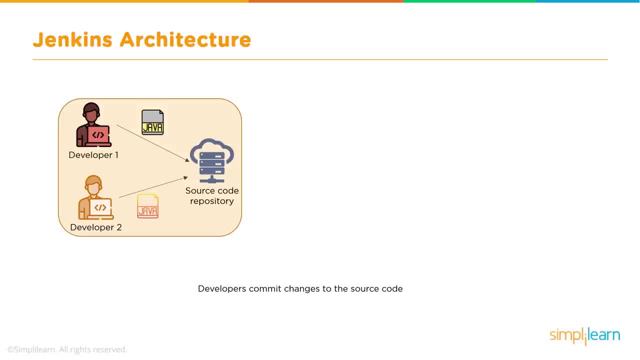 the developers are doing and submitting that code to a source code repository and then from then, Jenkins is your continuous integration server and it will then pull any code that's been sent to the source code repository and will run tests against it. they'll use a build service such as maven to actually then. 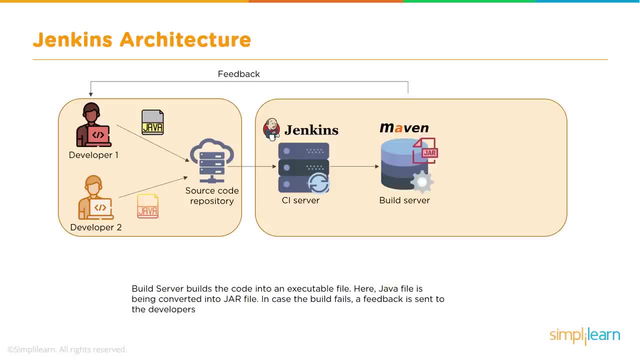 build the code and every single stage that we have that Jenkins manages. there are constant tests so, for instance, if a build fails, that it feedback is sent right back to the developers so that they can then change their code so that the build environment can run effectively. the final stage is to 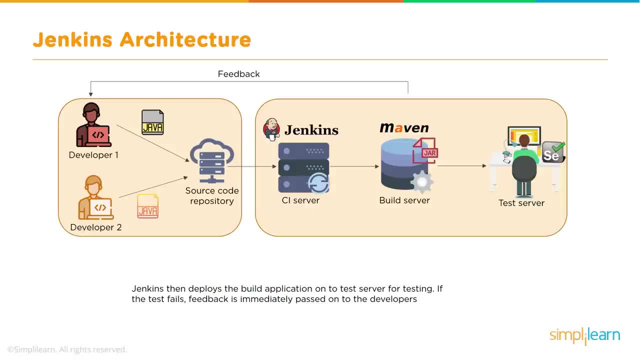 actually execute specific test scripts, and these test scripts can be written in selenium. so it's probably good to mention here that both maven and selenium are plugins that run in the Jenkins environment. so before we were talking about how Jenkins can be extended with plugins, maven and selenium are just two very popular examples of how you can. 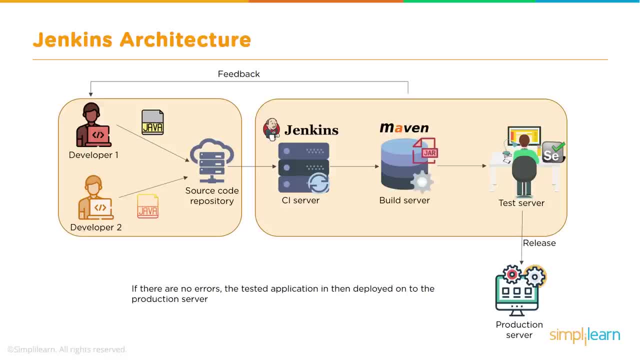 extend the Jenkins environment. the goal to go through this whole process- again, it's an automated process- is to get your code from the developer to the production server as quickly as possible, have it fully tested and have no errors. so it's probably important to at this point to mention one piece of information around the Jenkins. 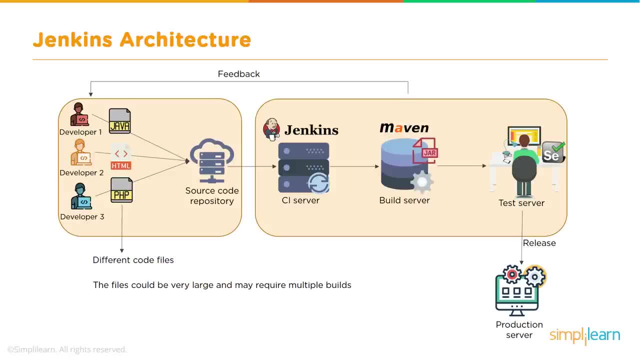 environment that if you have different code builds that need to be managed and distributed, this will require that you need to have multiple builds being managed. Jenkins itself doesn't allow for multiple files and builds to be executed on a single server. you need to have a multiple server environment with running. 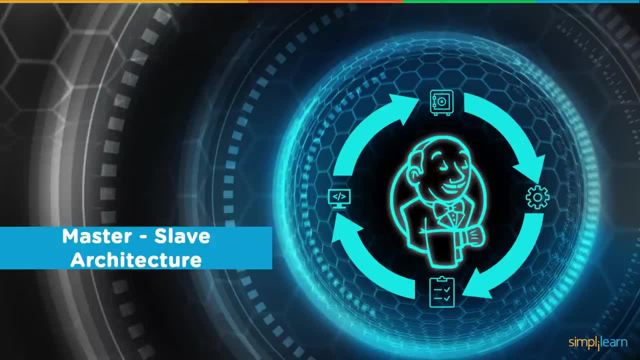 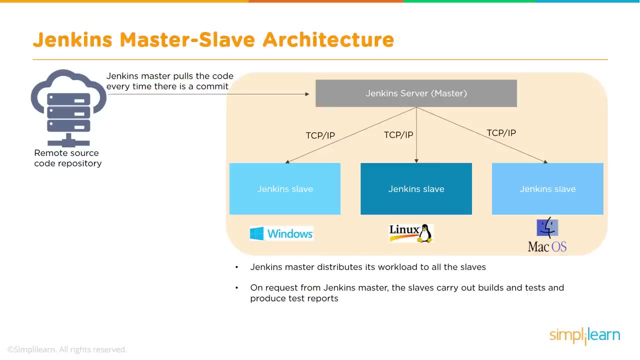 different versions of Jenkins for that to be able to happen. so let's talk a little bit about the master-slave architecture within Jenkins. So what we have here is an overview of the master-slave architecture within Jenkins. On the left hand side is the. 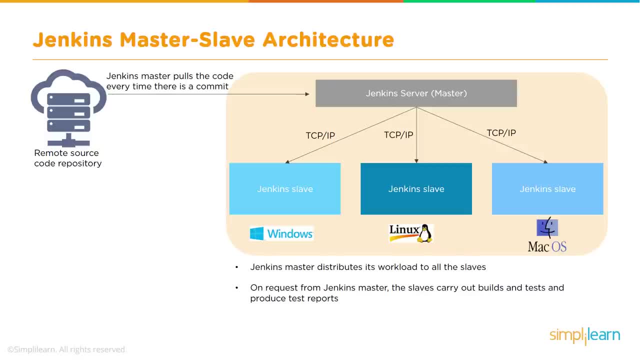 remote source code repository, and that remote source code repository could be github, or it could be team foundation services or the new Azure DevOps code repository, or it could be your own git repository. The Jenkins server acts as the master environment on the left hand side, and that master environment 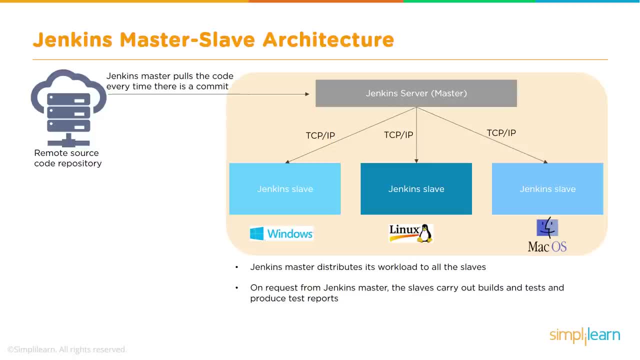 can then push out to multiple other Jenkins slave environments to distribute the workload, so it allows you to run multiple builds and tests and production environments simultaneously across your entire architecture. Jenkins slaves can be running the different build versions of the code for different operating systems and the server master is controlled off-the-cuff��, over-the-c, Colonel, and never contain architecture. The j dell officeツ可能 moving into an WINHU, and in fact we've planned to like wake up in the teller Controlling how each of those builds operate. 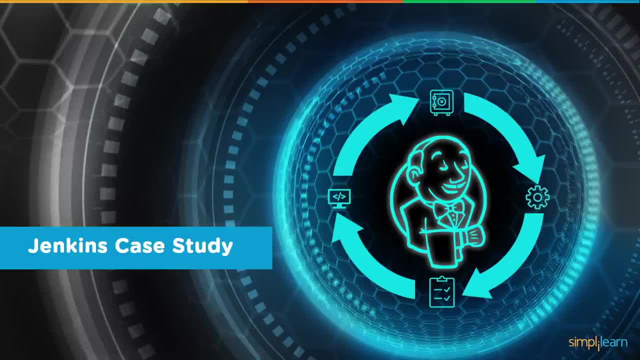 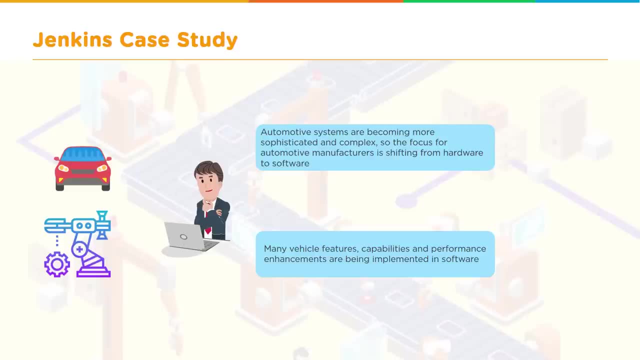 So let's step into a quick story of a company that has used Jenkins very successfully. So here's a use case scenario. over the last 10 or 15 years there has been a significant shift within the automotive industry, where Manufacturers have shifted from creating complex hardware to actually creating software. 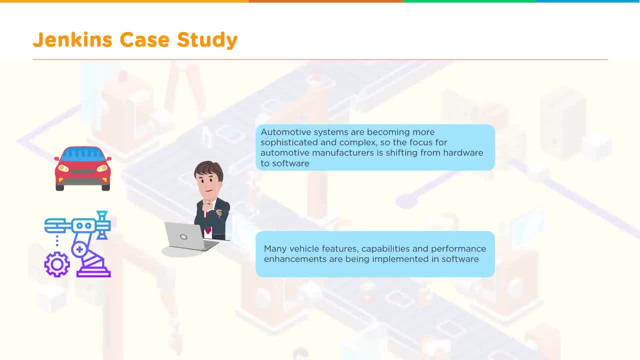 We've seen that with companies such as Tesla and where they are creating software to manage their cars. we see the same thing with companies such as General Motors with their OnStar program, and Ford just recently have rebranded themselves as a technology company rather than just a. 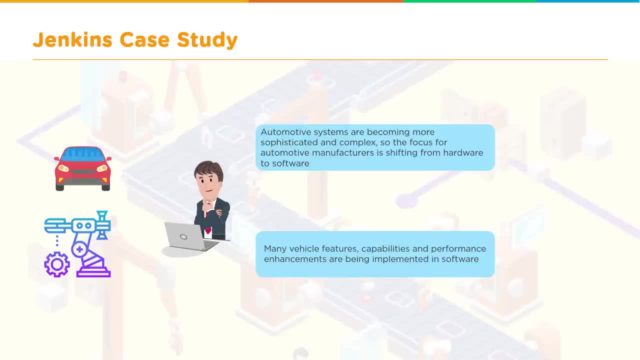 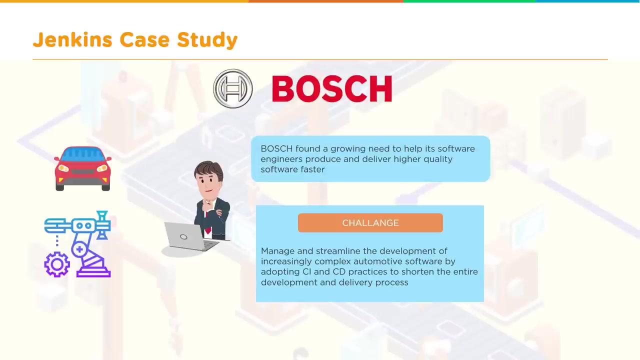 Automotive company. what this means, though, is that the software within these cars is becoming more complex and requires more testing to Allow more capabilities, enhancements, to be added to the core software, So Bosch is a company that specifically ran into this problem, and their challenge was that they wanted to be able to 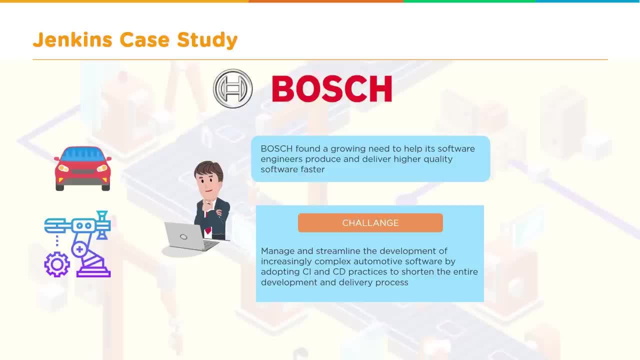 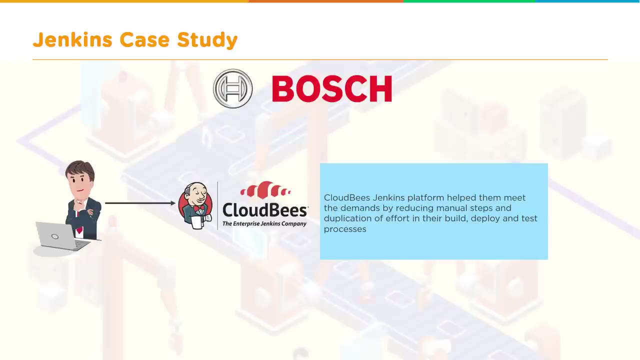 streamline the increasingly complex automotive software by adopting continuous integration and continuous delivery best practices, with the goal of being able to delight and exceed the customer expectations of the end-user. So Bosch has actually used cloud bees, which is the enterprise Jenkins environment, so to be able to reduce them the number of manual steps, such as building, deploying and testing. Bosch has 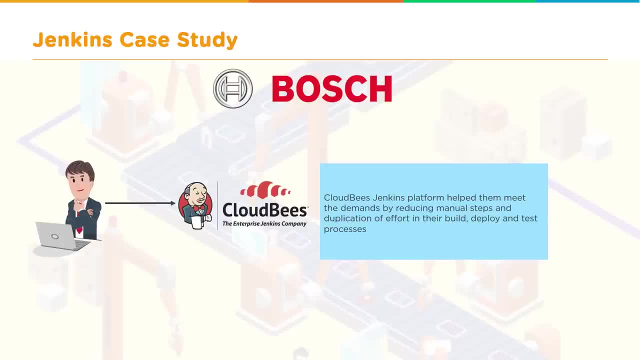 introduced. the use of cloud bees from Jenkins- and this is part of the enterprise Jenkins platform- has significantly helped improve the efficiencies throughout the whole software development cycle, from automation, stability and transparency, because Jenkins becomes a self auditing Environment. now the results have been tangible. Previously it took three days before a build process could be done, and now it's taken that same three-day process and reduced it to less. 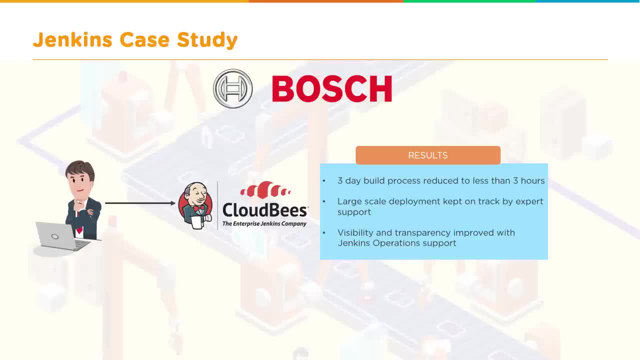 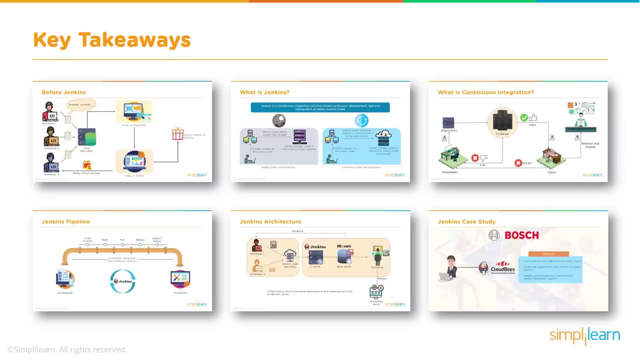 than three hours. that is significant. large-scale deployments are now kept on track and have expert support, and there is clear visibility and transparency across the whole of the industry operations through using the Jenkins tools. So some key takeaways from this presentations. first of all, we describe the developer hell that you may be in.